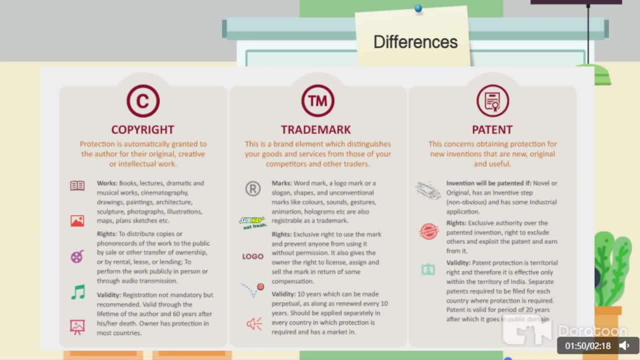 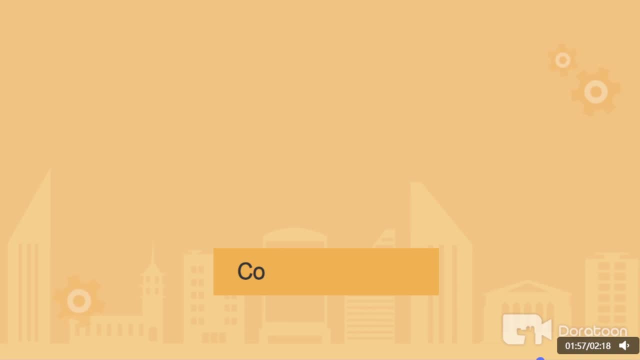 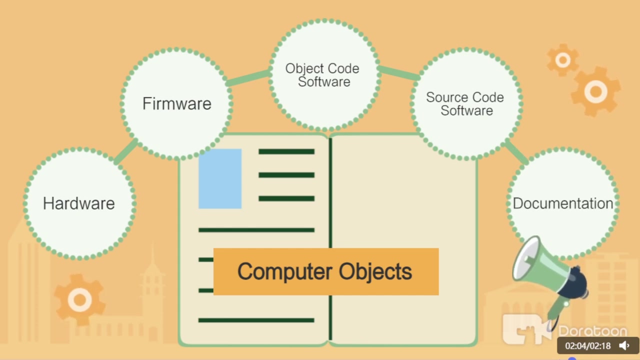 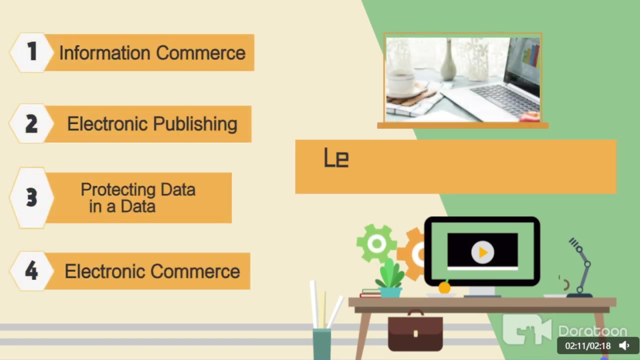 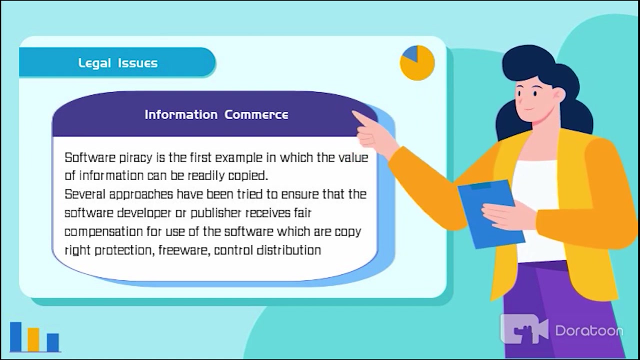 Sources from LegalWiz. Protection for computer objects could be Hardware, Firmware, Object code, software, Source code, software Documentation. Legal issue relating to information are Information commerce, Electronic publishing, Protecting data and a database. Electronic commerce- Software piracy- is the first example in which the value of information can be readily copied. 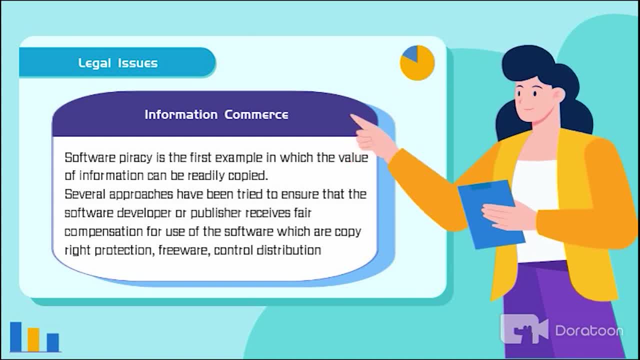 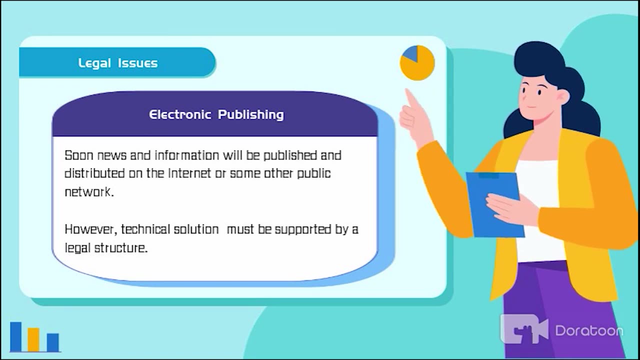 Several approaches have been tried to ensure that the software developed or our publisher receives fair compensation for use of the software, which, or copyright protection, freeware, controlled distribution, Soon, news and information will be published and distributed on the internet or some other public network. 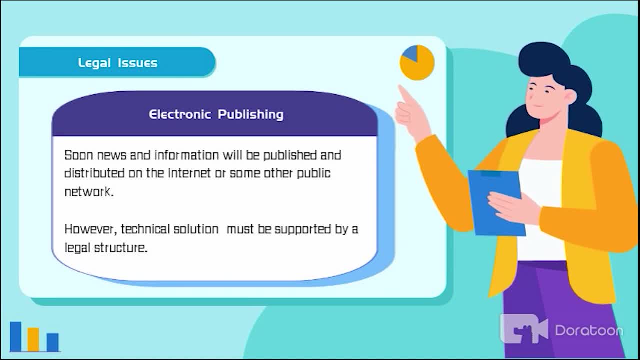 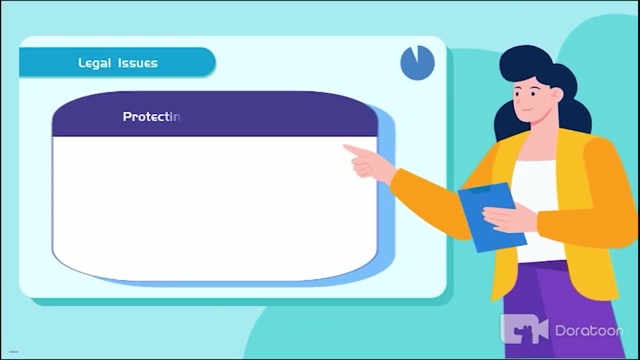 However, technical solution must be supported by a legal structure. The courts have difficulty interpreting protection laws for application to data. The courts have difficulty interpreting protection laws for application to data. The courts have difficulty interpreting protection laws for application to data Protected document. software is one of the first systems in Asia's soon running söyed with computer cooperation. 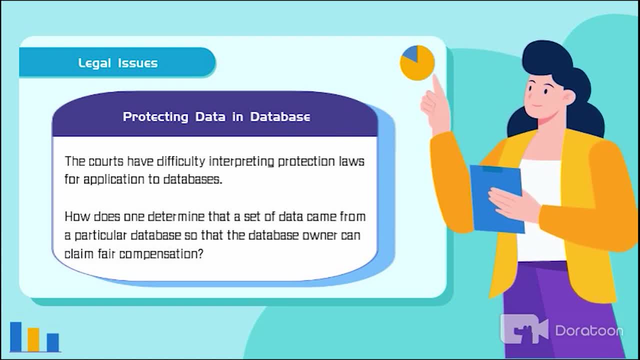 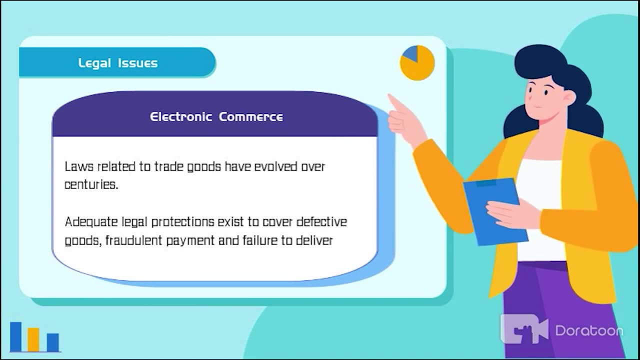 How does one determine that a set of data came from a particular database so that the database owner can claim fair compensation? That is for us to find out The words don'tcein. Laws related to trade goods have evolved over centuries. Equally safe legal protection exists for incorrectly 불�URECTING, misunderstood words. 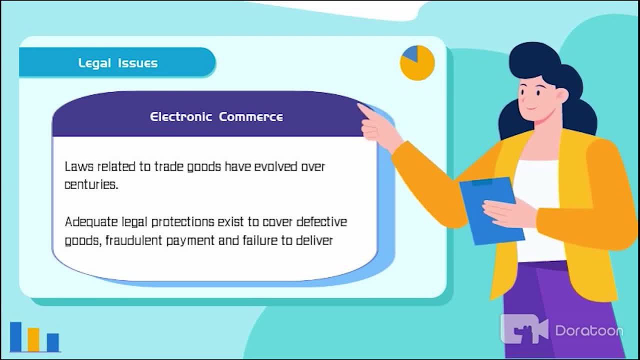 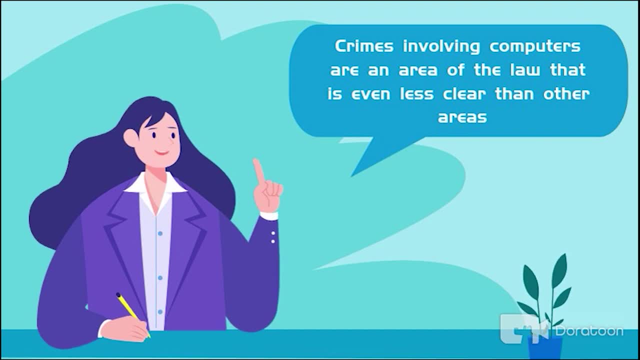 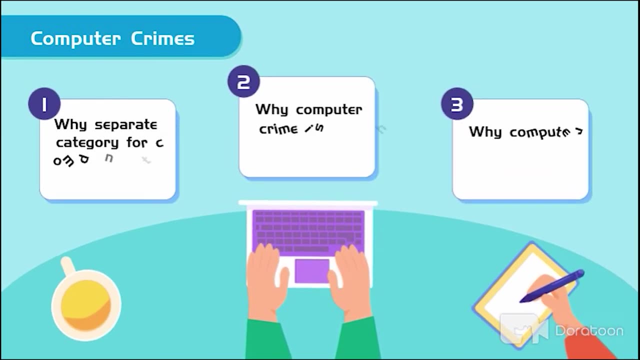 Produlent payment and failure to deliver, Crimes involving receiving negative Thing. Crimes involving computers are an area of the law that is even less clear than other areas. There are few issues to be discussed here. Why separate category for computer crimes? Why computer crime is hard to define? Why computer crime is. 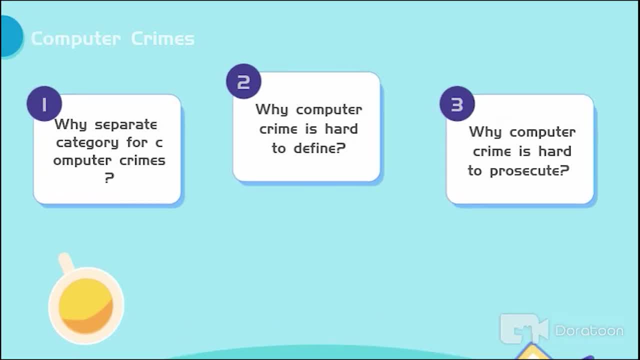 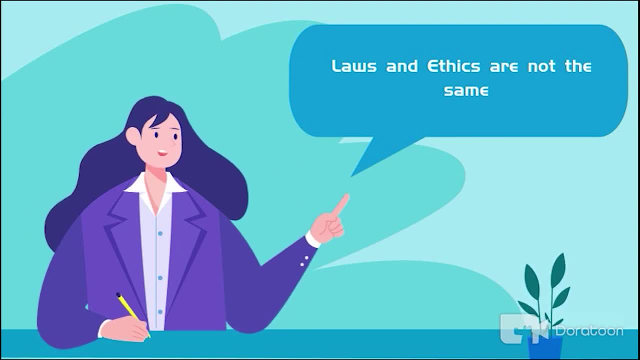 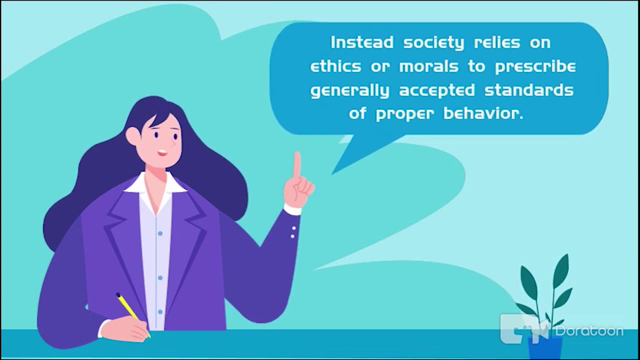 hard to prosecute. Laws and ethics are not the same. Law is not always appropriate to deal with issues of human behavior. Instead, society relies on ethics or morals to prescribe generally accepted standards of proper behavior. Thanks for watching.